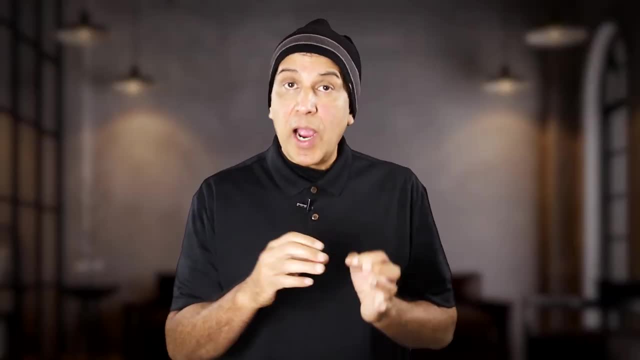 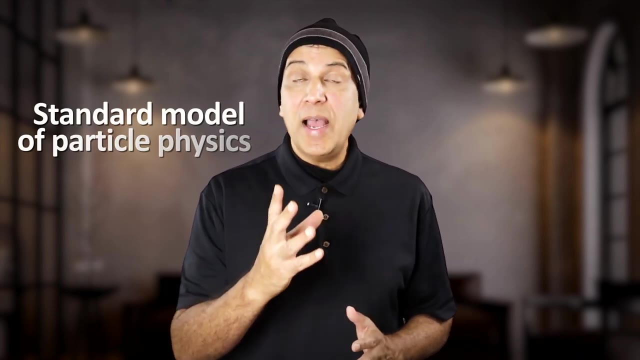 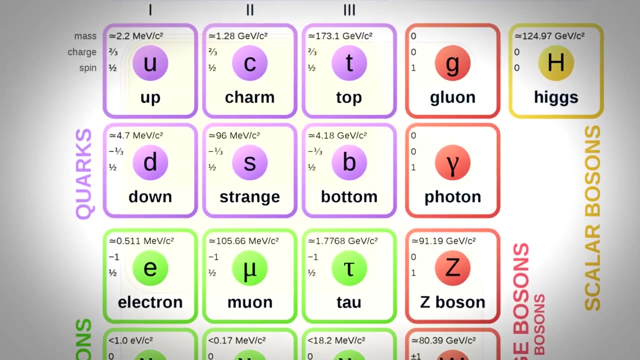 as far as we know, The best theory we have to describe these fundamental particles and how they interact with each other is called the standard model of particle physics. This is the best, most accurate theory we have today And this is what you'll find if you google the standard model. 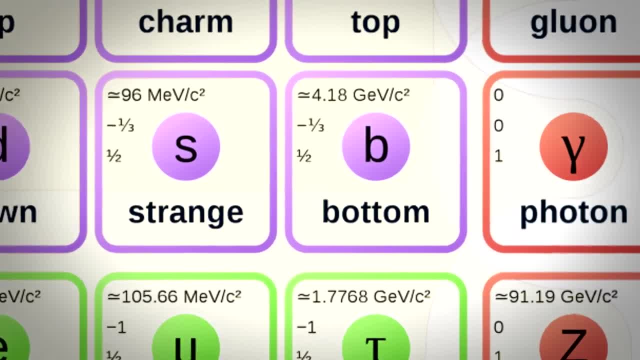 This table can be thought of the same way as the periodic table of elements in chemistry, listing all the known atoms we know of. Although this is what you see in the periodic table of elements in chemistry, Although this is what you see in the periodic table of elements in chemistry, Although this is what you see. 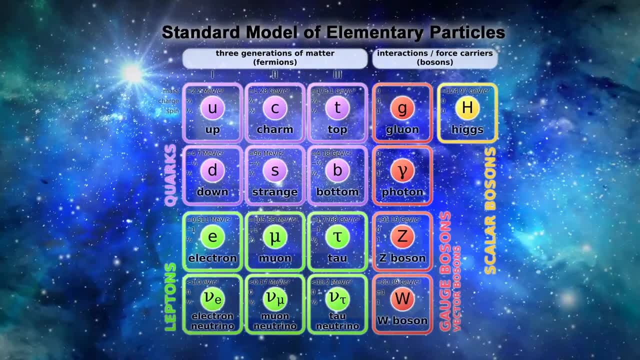 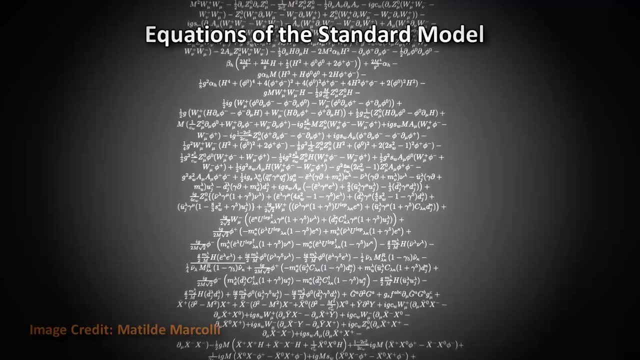 in the periodic table of elements. in chemistry, Although this is what you see, the standard model isn't just the particles shown here, but is an umbrella term that denotes everything we know about the microscopic world, the world that operates by the rules of quantum mechanics. 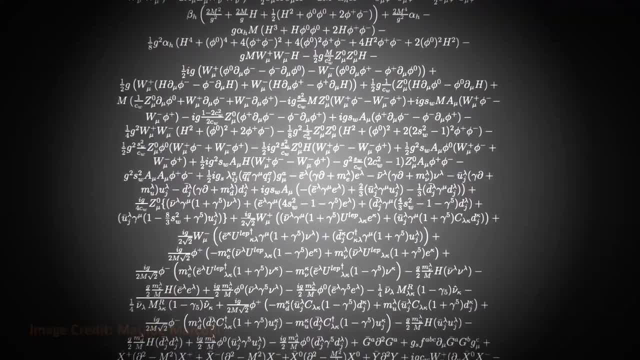 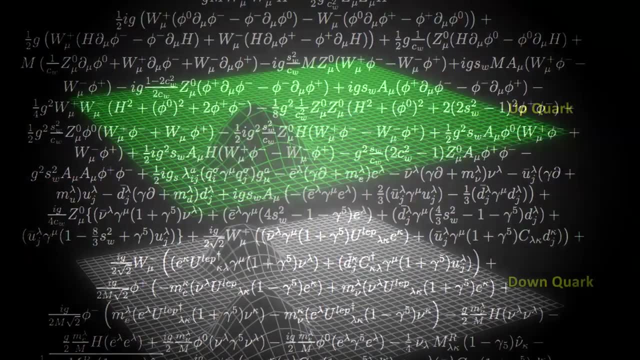 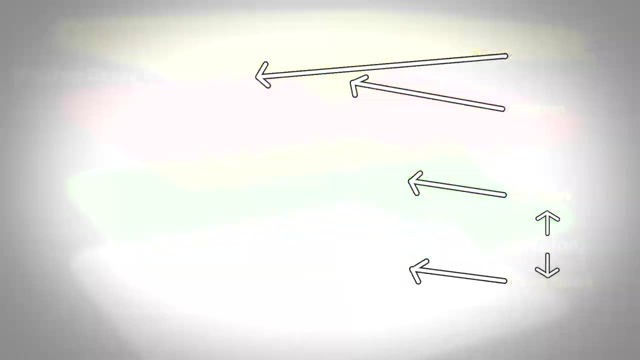 It encompasses the sets of rules about how the fundamental particles we know of interact with each other and how these interactions are mediated by the different fundamental forces. It's, more precisely, a collection of quantum field theories describing the strong, weak electromagnetic force, and more. In this video I'll show you. 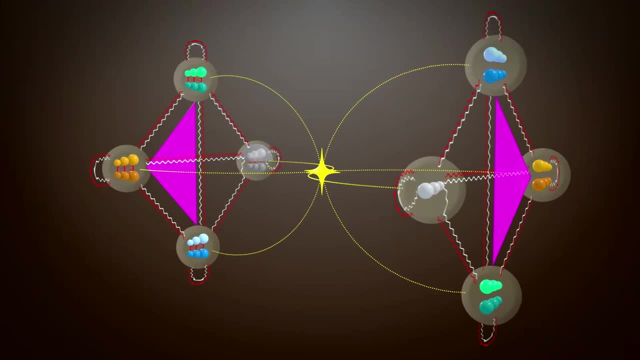 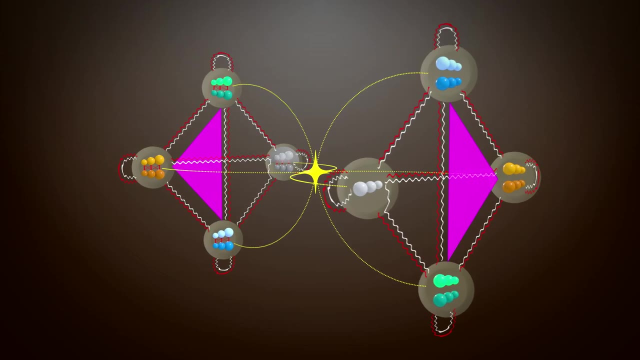 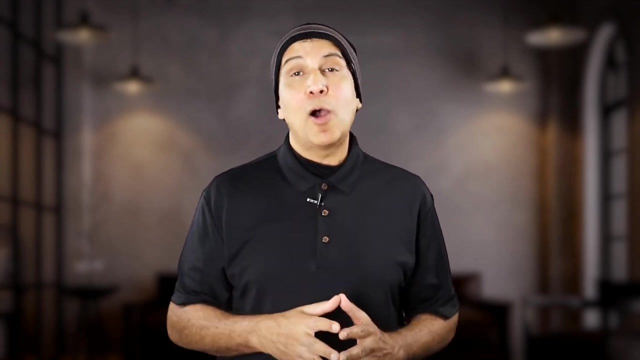 a different way to visualize the standard model, such that you can more clearly see not only the uniqueness of each particle, but also how they interact with each other and how the fundamental forces and the Higgs boson connect everything to everything else. In this way, I hope to show you visually how particle physics works. 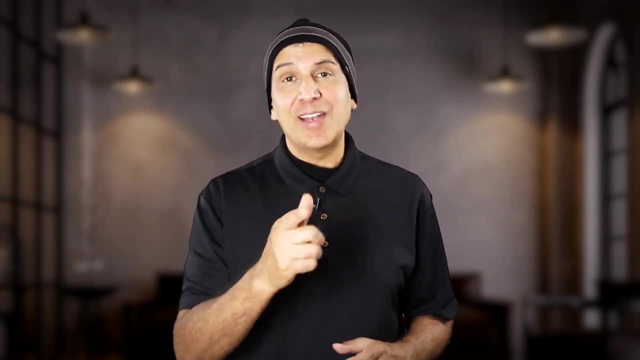 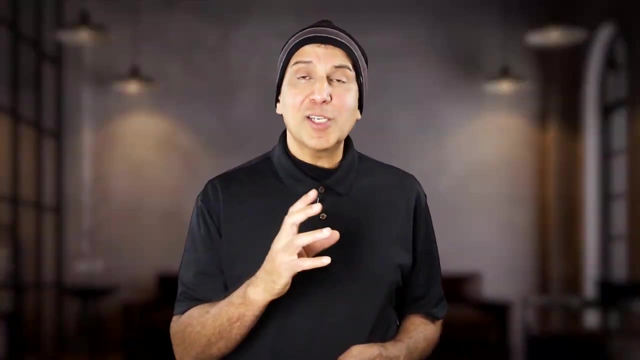 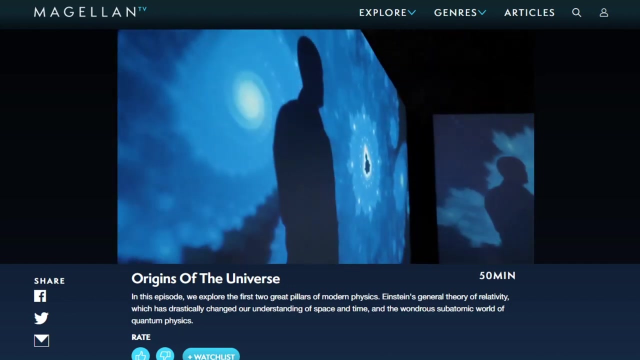 as best we understand it today, And that's coming up right now. Some of you might wonder what inspires me to make videos on a particular topic. One documentary that inspired me was a new one on MagellanTV today's sponsor, called Origins of the Universe. It's part of a brand new series called Jim. 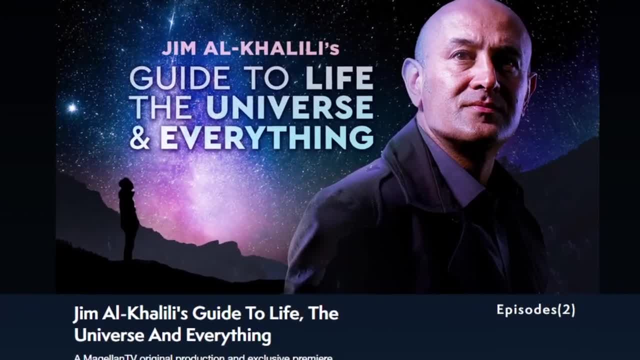 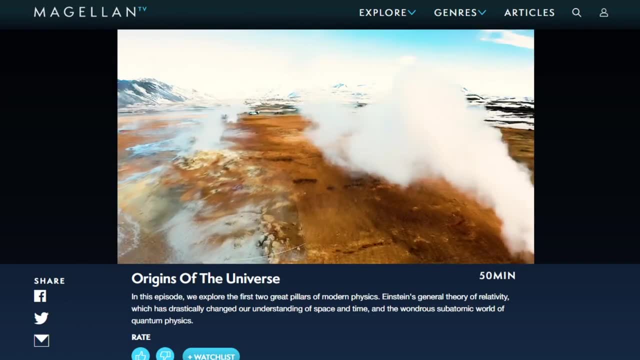 Al-Khalili's Guide to Life, the Universe and Everything. This new series will cover cosmology, quantum physics and quantum biology. In the Origins of the Universe episode I was inspired by Jim's simple yet in-depth examination of quantum mechanics in the 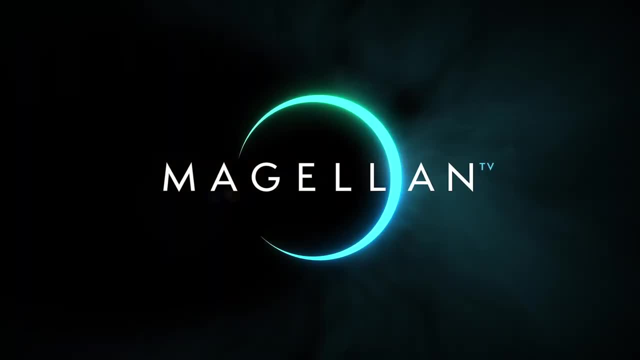 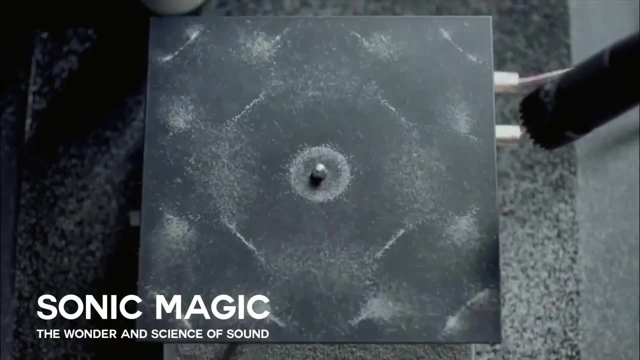 subatomic universe. I highly recommend you check out this new series on MagellanTV. It's a new kind streaming documentary service created by the filmmakers themselves. You'll find not only fascinating science videos, like the ones from Jim Al-Khalili, but also on subjects like history. 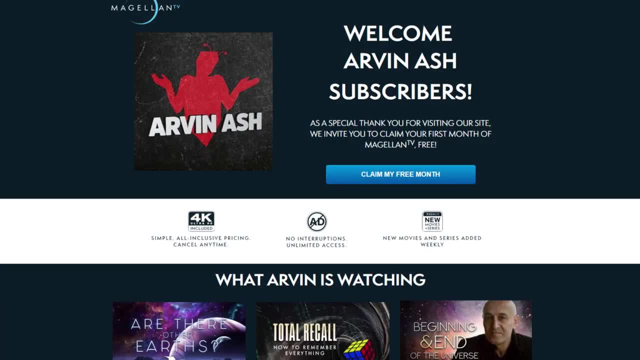 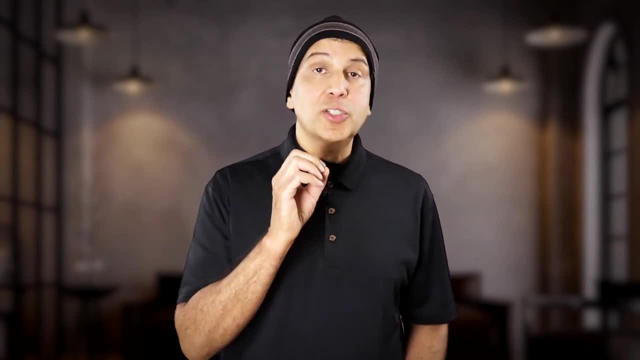 nature and travel. If you sign up for Magellan using the link in the description, you'll even get a free one month trial, So be sure to take advantage of this by clicking the link in the description. First, I want to give credit to theoretical physicist Chris Gray, who is a 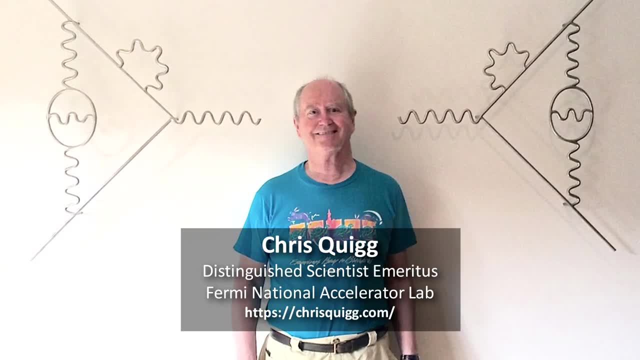 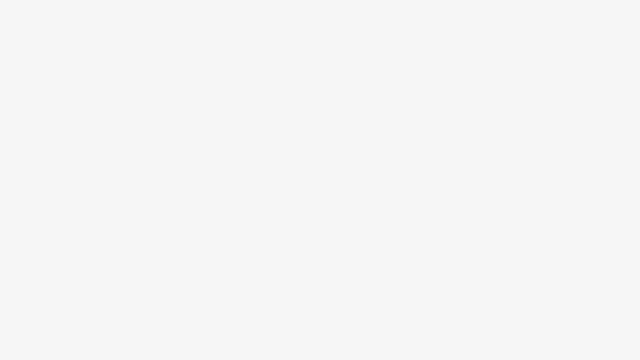 distinguished scientist emeritus at Fermilab. He's the one that conceptualized the visualization I'm talking about. You can visit his website at the link in the description. Now let's start by throwing away the table of the standard model and begin with a clean slate. 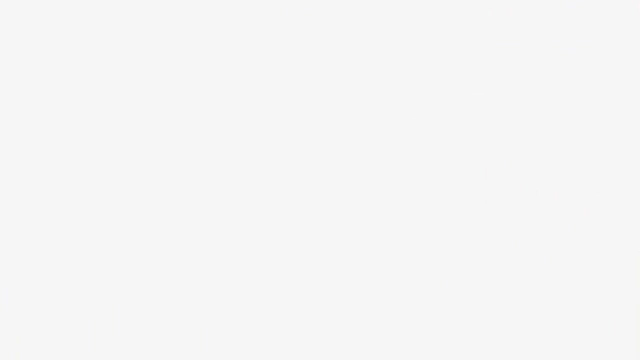 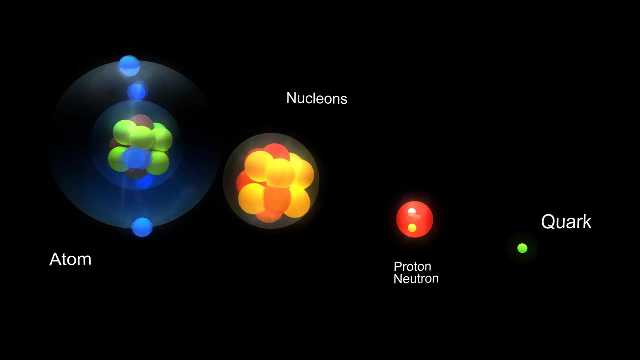 We'll start with nothing and go step by step while exploring the standard model. First, let's build an atom. To do this, we need quarks. The nucleus of atoms contains neutrons and protons. These are made of either a combination of two up and one down quarks. 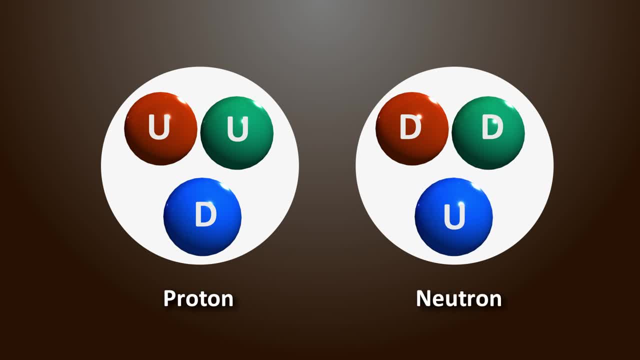 in the case of the proton, or two down and one up quark for the case of the neutron. These quarks come in two values of electrical charge. The up quark has a charge of plus two thirds and the down quark has a charge of negative one third. So the total charge of 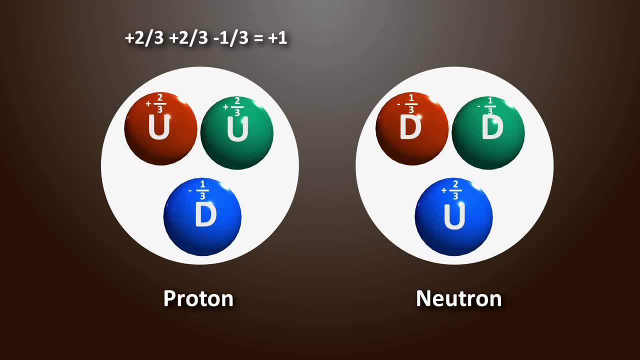 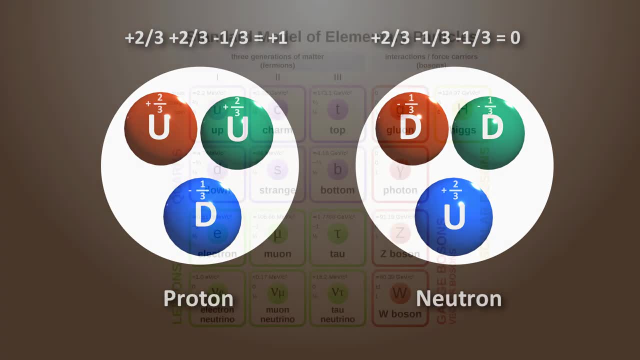 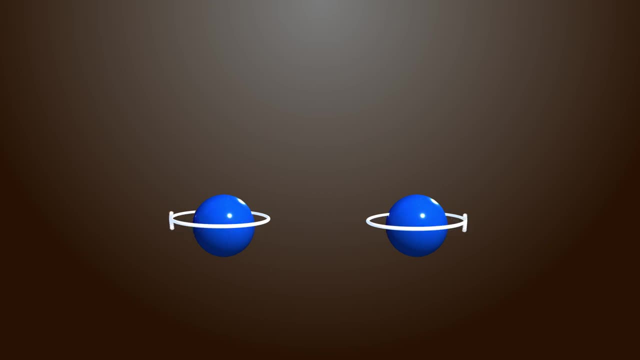 the proton is plus one. if you add up the charges from two up and one down quark. Similarly, the total charge of the neutron adds up to zero. We have two classes of matter particles in the standard model: leptons and quarks. Matter particles have this special property of spin. 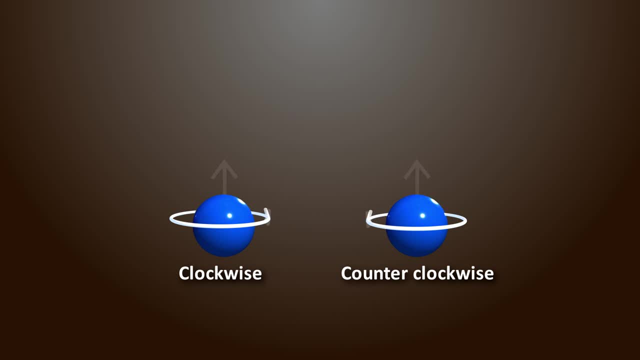 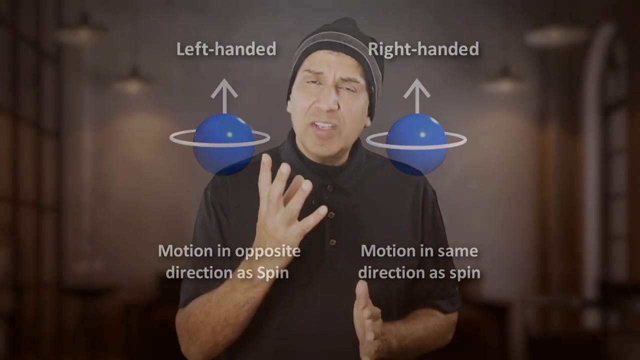 they can spin clockwise or counterclockwise And depending on what way the particle spin is in relation to its direction of motion, it is classified as either a right or left-handed particle. Quarks come in both types, left-handed and right-handed. Now, this aspect of handedness. 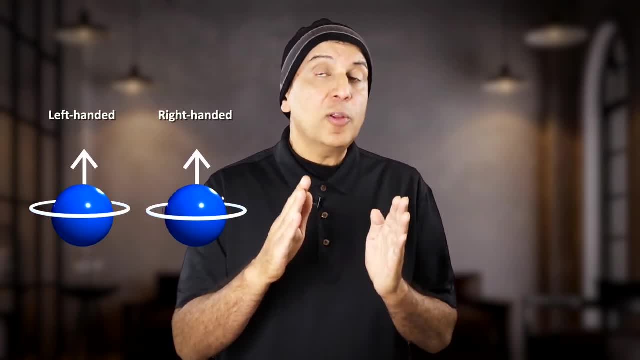 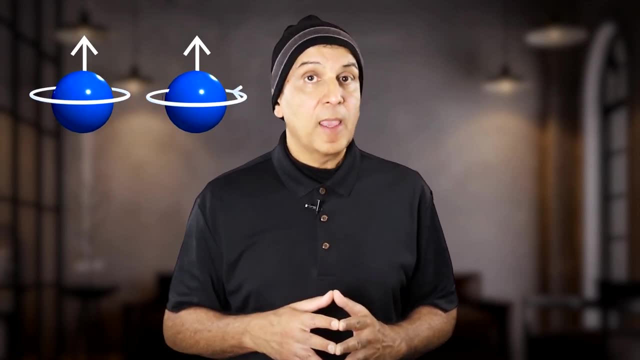 is very important because it turns out to be crucial for how the particles interact. This is something that is completely omitted from the typical representation of the standard model. Left-handed up and down quarks can transform into each other via an interaction of one of the 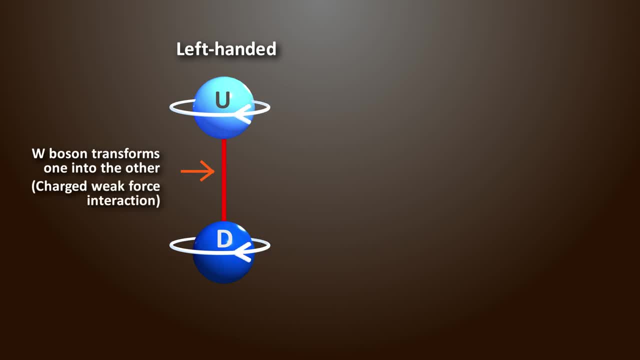 fundamental forces of nature called the weak force. This is called a charged weak force interaction and is mediated by a W plus boson, which has a charge of plus one, or a W minus boson, which has a charge of minus one. This line represents the W boson charged interaction. 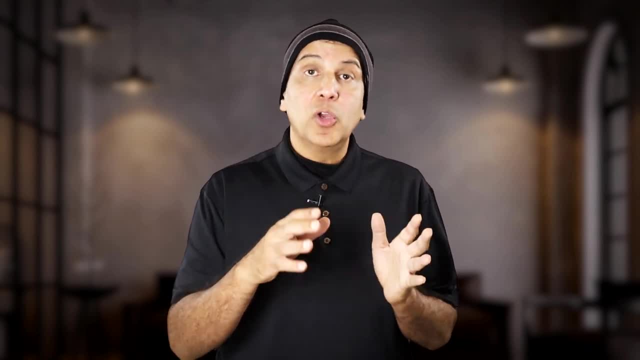 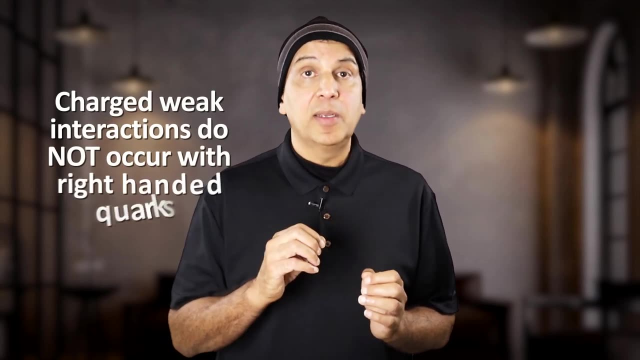 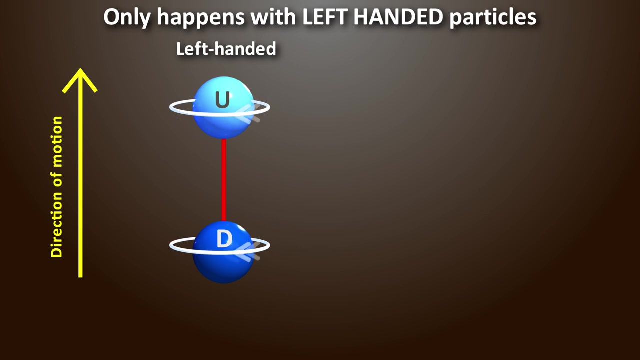 Now, for some unknown reason, nature turns out to not treat left and right-handed particles the same way, because this interaction does not happen with right-handed quarks. It is not known why. This means that right-handed quarks cannot change into other quarks and remain the same particle always. There is no charged weak interaction. 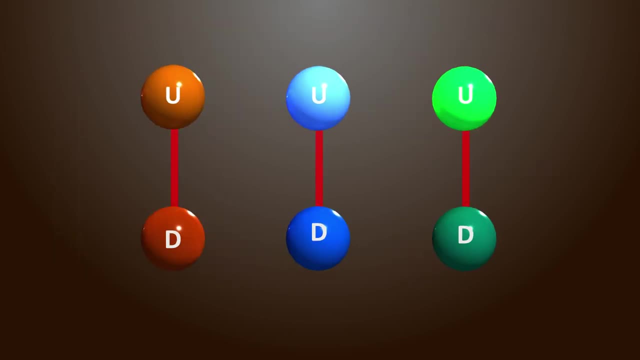 between right-handed particles at all. The quarks also have another charge called color charge or, more precisely, each type of quark exists in three different colors: red, blue and green. The color charge allows quarks to interact via another fundamental force of nature. 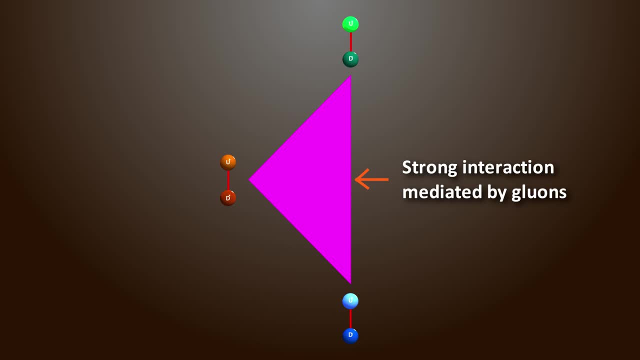 the strong force. The strong force is mediated by another boson called the gluon. This strong force interaction allows three quarks of different colors to be bound together to make a proton or neutron in the nucleus of atoms. We can represent this force by showing a triangle. 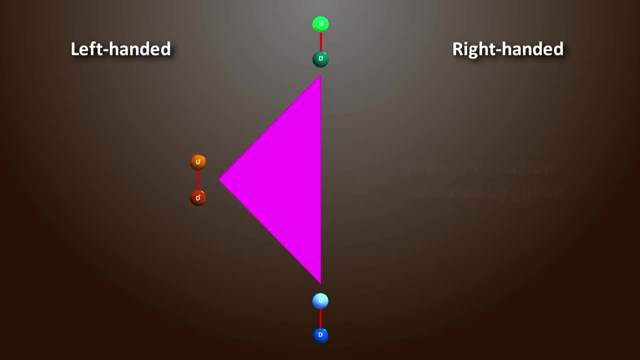 between the different colors. Note that the triangle is the same for left and right-handed particles, because the strong force on the right-hand side is the same for the left-hand side. The strong force on the left-hand side is the same for the right-hand side because the strong force on 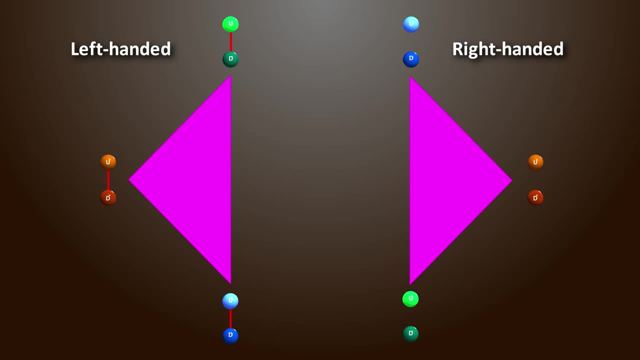 the right-hand side is the same for the left-hand side, Unlike the weak force, does not discriminate between left and right-handed particles. It treats both types of particles the same way. The colors of these quarks are constantly changing by emitting and absorbing gluons, But all 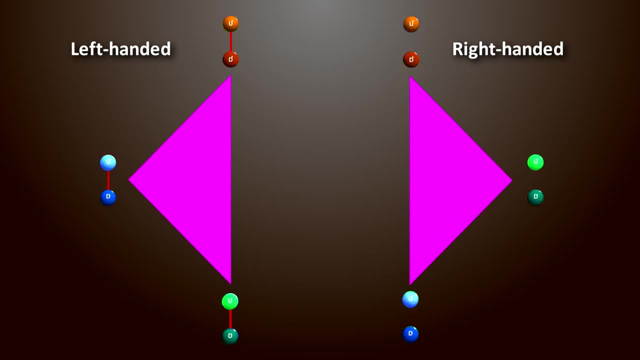 three quarks must be of the three different colors- red, green and blue- to make a neutral or colorless charge. Any two of the three quarks can't be the same color at the same time. So far we have the following for quarks: There are up and down quarks. These quarks can be further. 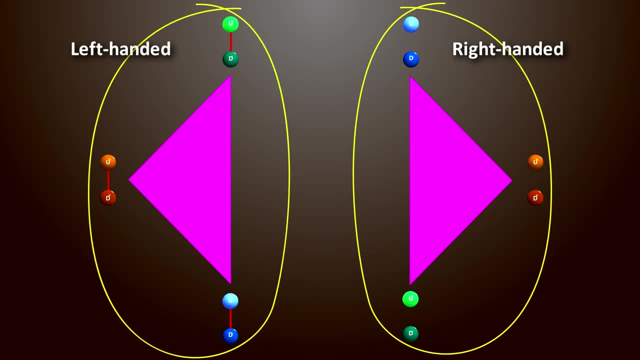 into two groups, depending on if they are right or left-handed. In each group there are three colors of each quark. So as of now, we have 12 different quarks, 6 different up quarks and 6 different down quarks. Again, looking at the standard table of the standard model, you might be fooled that there 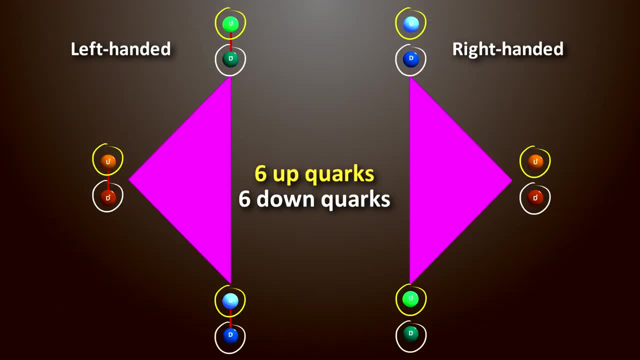 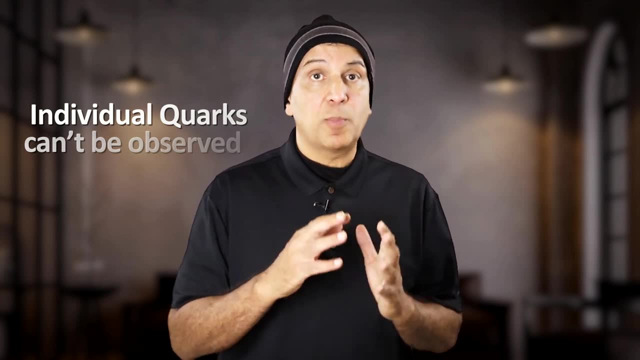 is just one up and one down quark, but there are really 12, as shown here. You should know that quarks by themselves can never be observed. The theory tells us that only colorless particles can be observed. A colorless particle can only be observed if it is observed by a single particle. 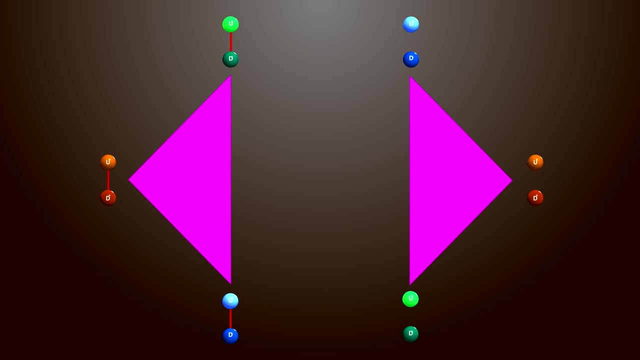 The theory tells us that only colorless particles can be observed. A colorless particle can only be formed in one of two ways. You can either combine quarks of three different colors- red, green and blue- to make a neutral color combination, like in neutrons and protons. 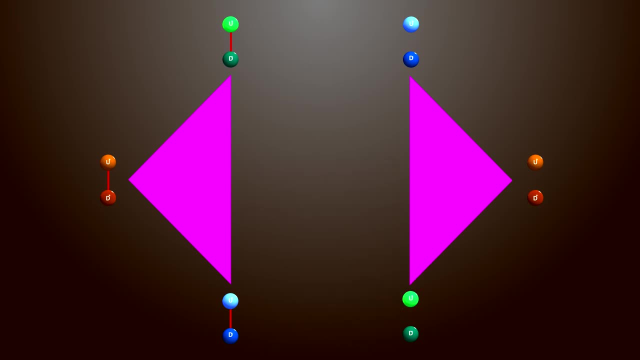 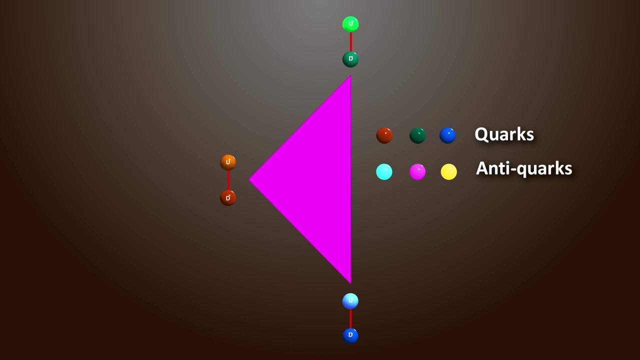 which can be observed. Or you can combine quarks and anti-quarks. Yes, there are anti-quarks that carry an anti-color, So there are anti-red, anti-green and anti-blue anti-quarks. When a quark binds to an anti-quark, the particle that is formed is called a meson, which can be observed. 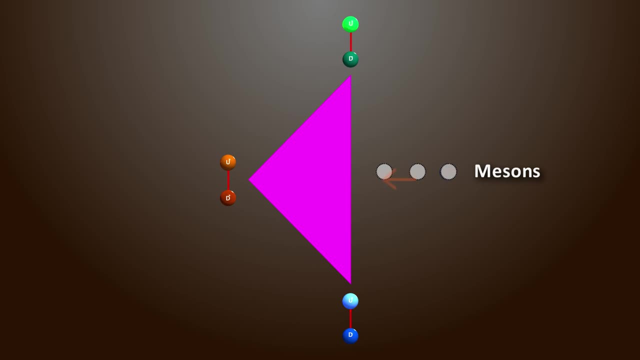 These color rules come from the strong force. The strong force is mediated by a particle called the gluon. Like glue, it binds quarks tightly together. There are actually 8 different gluons with different combinations of colors. Gluons act as a mechanism to transfer colors from one quark to. 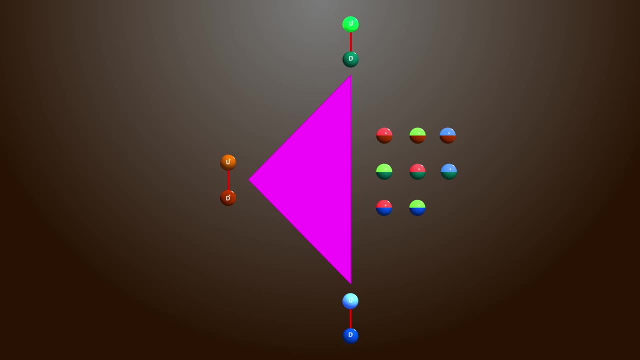 another. This transfer of colors is what binds quarks together. I made a very detailed video on how this happens using Feynman diagrams, if you are interested in knowing the mechanics of this. The gluons act as a mechanism to transfer colors from one quark to another. The gluons act as a 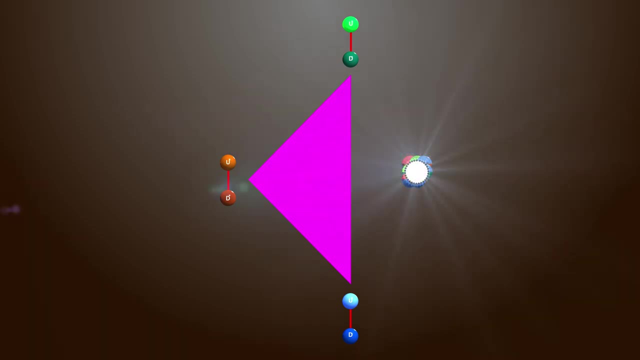 mechanism to transfer colors from one quark to another. These are not colorless but theoretically you could combine them such that you can make a composite ball of gluons that is colorless and could be detectable, But so far no one has ever detected a glue ball. 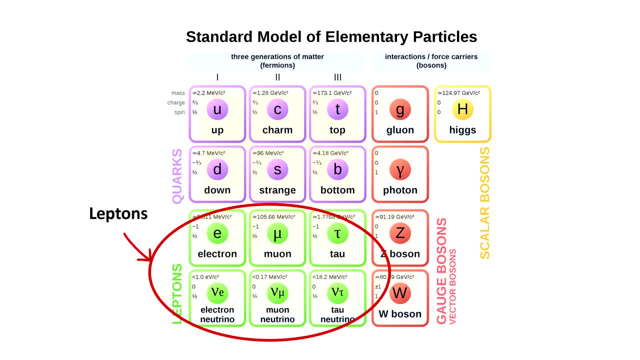 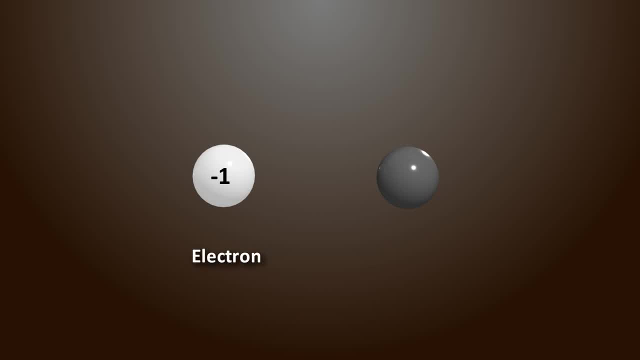 Now let's look at the second class of matter, particles called leptons. Again, we have two types of leptons in terms of charges. We have the electron with a charge of negative one and the neutrino with a neutral charge of zero, Like with. 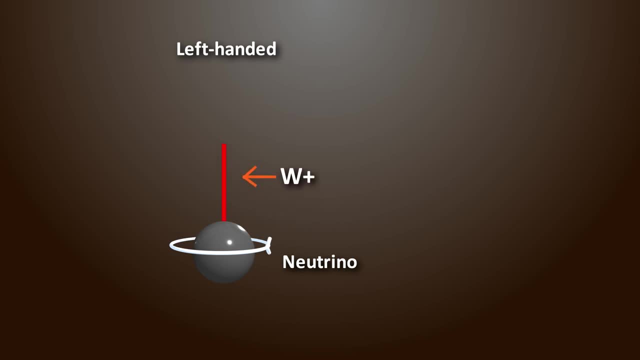 left-handed up and down quarks. the charged weak force can transform left-handed electrons and neutrinos into each other too, via the exchange of the W boson. While both left-handed and right-handed electrons exist, when it comes to neutrinos, for some reason only left-handed. 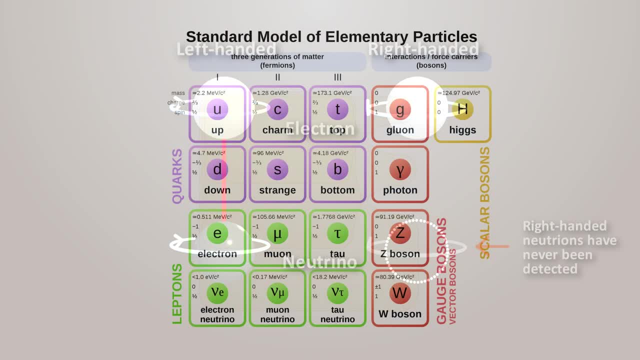 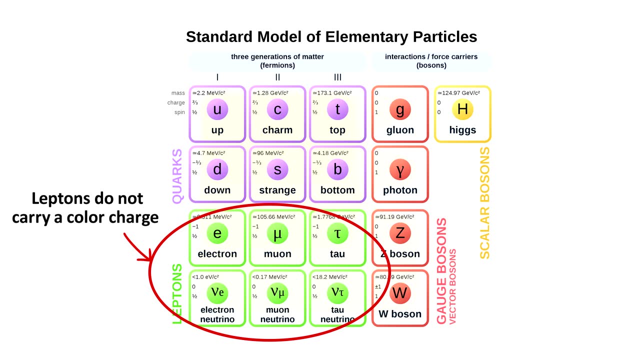 neutrinos exist. Right-handed neutrinos have never been detected. Unlike quarks, leptons do not have any color charge, and so they are not affected by the strong force. This lack of color charge is the main distinction between leptons and quarks. 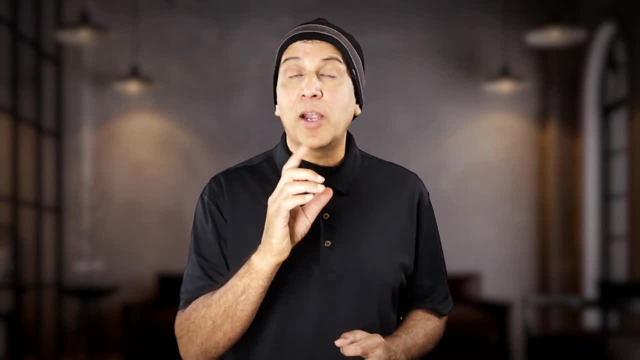 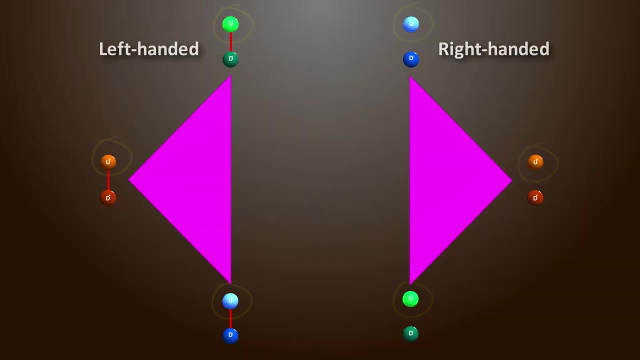 So with that let's do a quick summary of what we've learned about matter particles thus far. There are two classes of matter particles: quarks and leptons. For the quarks, there are six up quarks and six down quarks. They carry both electrical charge and color charge. 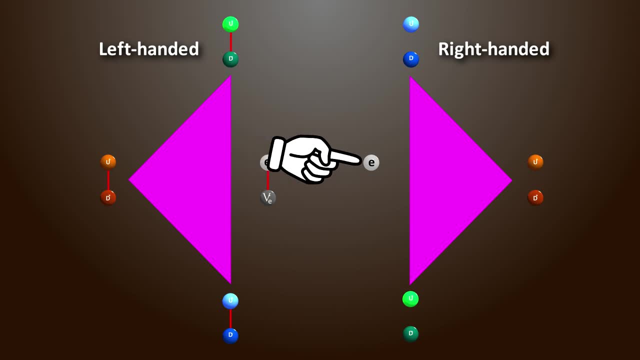 For leptons there are two electrons, left-handed and right-handed, and one neutrino, left-handed only. Electrons only carry electrical charge and do not have a color charge. Neutrinos do not carry any electrical charge or color charges. So to sum it up, we have 15. 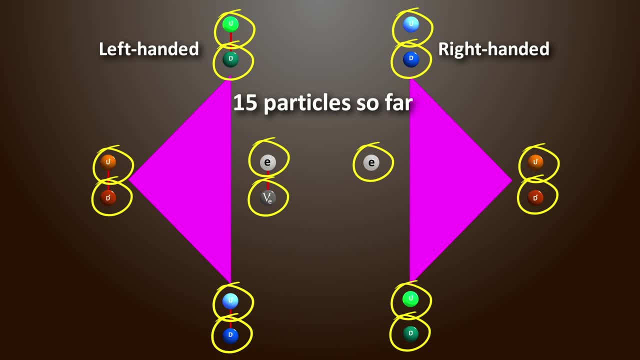 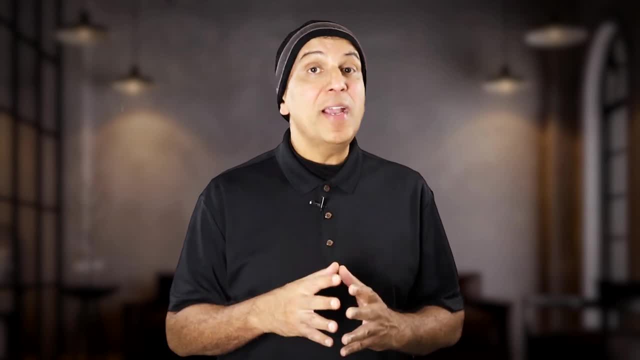 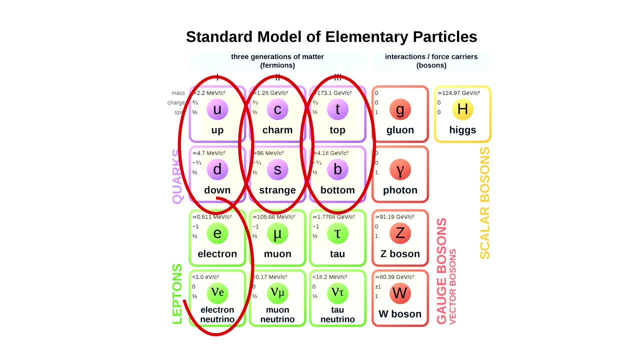 particles so far. Recall that physics is about explaining what we see and not about creating something that we decide. We just observe, We don't make the rules. I say this because, for some strange and unknown reason, the universe appears to contain what we call three generations of particles. What we have discussed so far is that the universe has three generations of particles. What we have discussed so far is that the universe has three generations of particles. What we have discussed so far is that the universe has three generations of particles. What we have discussed so far. 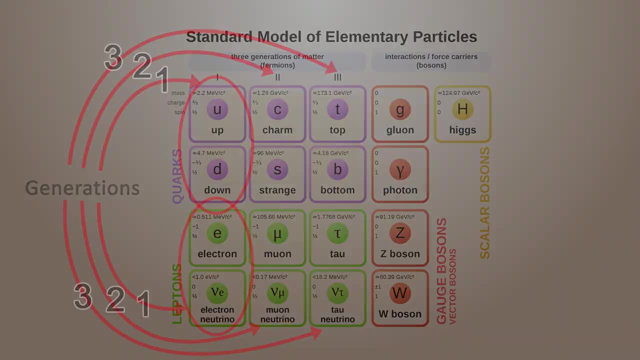 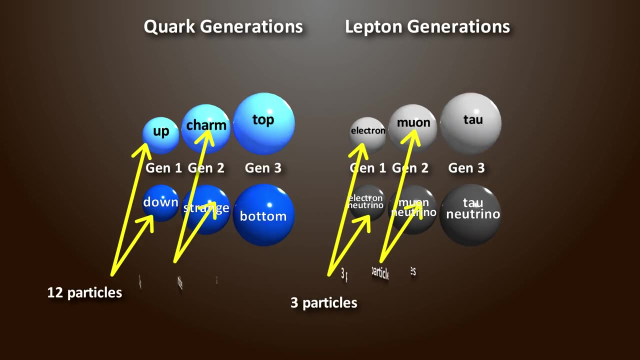 was only the first generation of matter particles, But there are two more generations. Each generation contains the same number of particles. Thus we get another 15 from the second generation and 15 more from the third generation. In total, we have 45 particles. The only difference between: 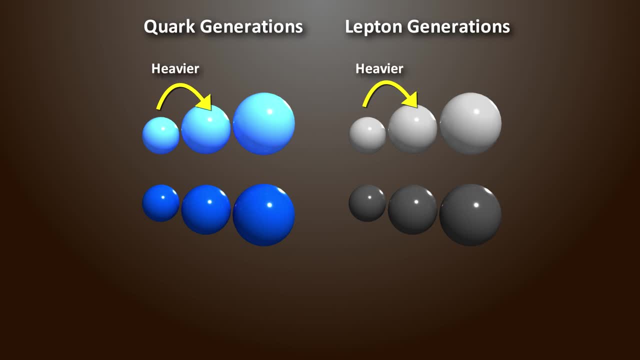 the generations is that the particles of generation 2 are heavier than generation 1, and the particles of generation 3 are even heavier than generation 2.. There is no other difference that we can tell. To this day, scientists have no clear understanding of why. 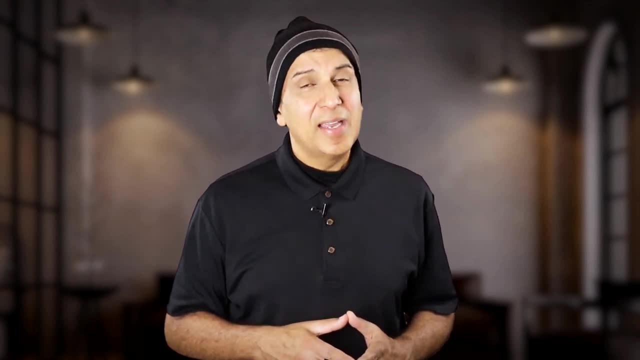 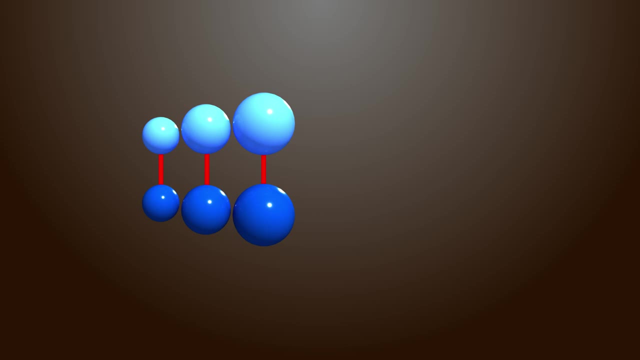 there are three generations, except the theory just works this way and the three generations match our observations. It turns out that left-handed quarks can not only transform between particles within the same generation but also across generations to a lower mass particle. So, for example, the charm quark, which is the heavier second generation version of the up quark, can decay. 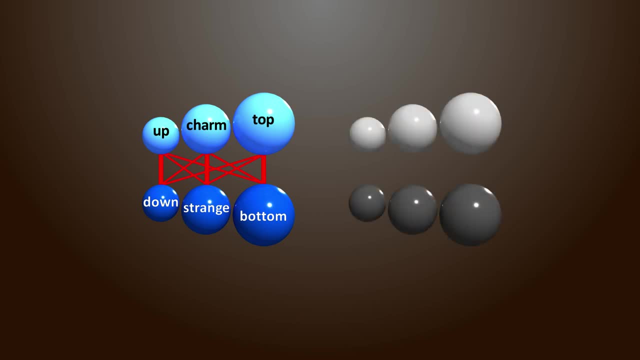 into a first generation, which is the heavier second generation version of the up quark, which is the heavier second generation version of the up quark, which is the heavier second generation version of the down quark. In terms of leptons, there is nothing in the theory that prevents them from transforming. 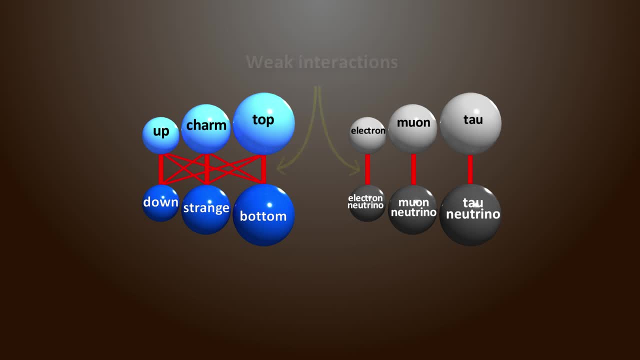 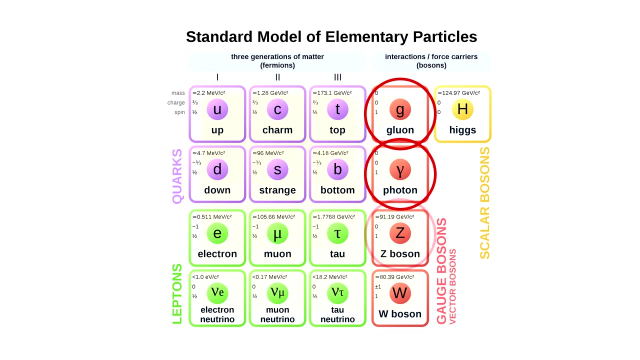 between particles of different generations, but so far this has never been observed. This is, however, an area of current research and there are signs that this kind of transformation could exist, but, as of right now, evidence shows that only quarks transform across generations. Let's move now to the non-matter particles, the bosons. 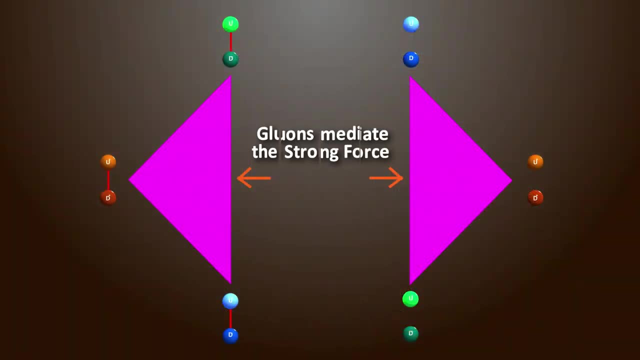 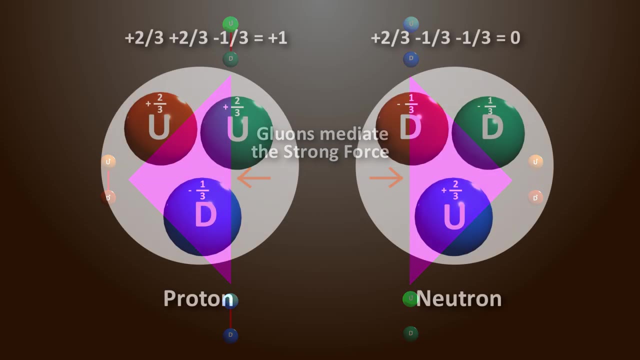 We discussed in some detail the strong force mediated by gluons which binds the quarks to together into composite particles such as neutrons and protons. We talked a little bit about the electrical charge, the fact that quarks have a charge of either two-thirds or negative one-third. 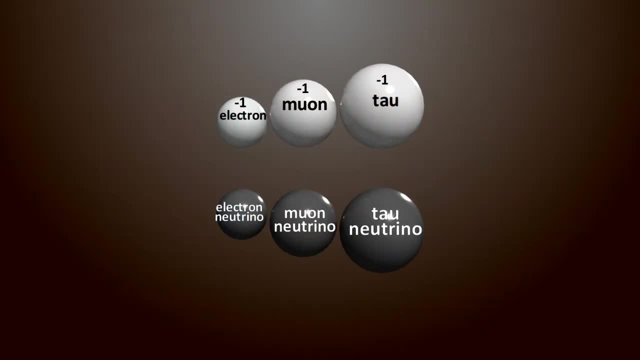 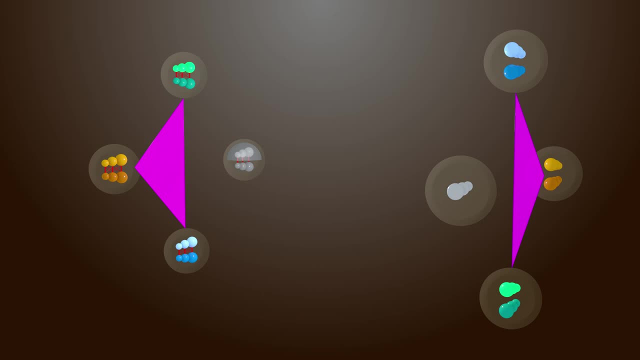 The electron and its heavier generations all have a charge of negative one, and all neutrinos are neutral, with a charge of zero. The force responsible for this charge is the electromagnetic force and it interacts with all matter particles except the three neutrinos. so we can draw a. 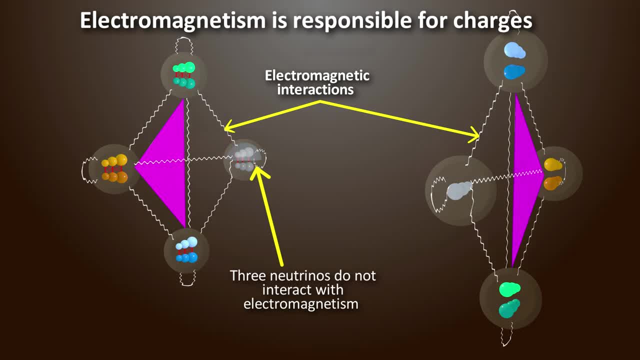 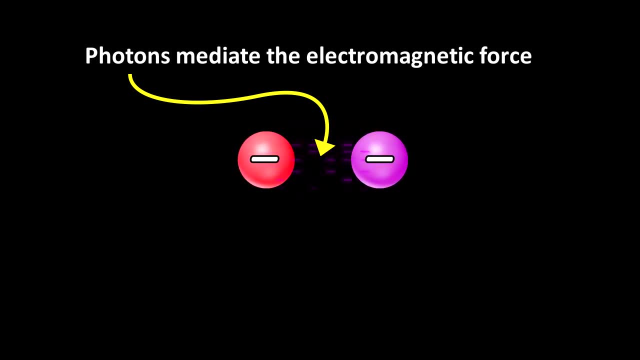 connection between all these particles. So let's look at the electromagnetic force. Just like the gluons mediate the strong force, photons mediate the electromagnetic force. In other words, the exchange of photons is what confers the electromagnetic force between two electrically charged objects. We also talked a bit about the weak force. 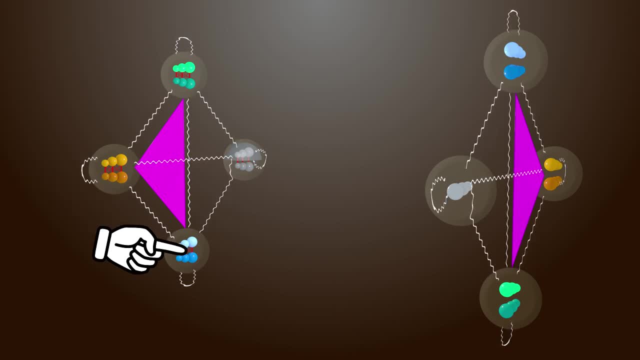 As I said earlier, only left-handed quarks can transform into one another via the weak force and only left-handed electrons and neutrinos can transform into each other via the weak force. And these interactions that change one particle to another are made possible by the change of the weak force and the change of the neutrinos. So let's look at the weak force. 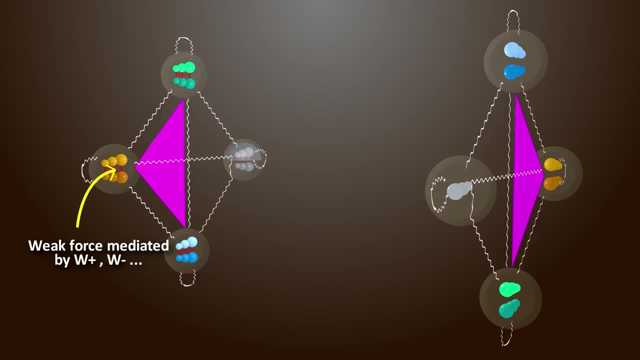 A third boson involved in weak interactions is the z-boson. However, it does not have any electrical charge. The exchange of a z-boson acts to only transfer momentum, spin and energy between particles, while leaving any other properties of interacting particles unaffected, Since there is 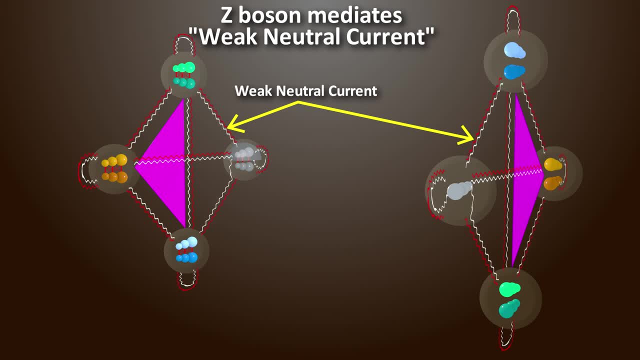 no transfer of electrical charge. the z-boson acts to only transfer momentum, spin and energy. This is referred to as a weak-neutral-current interaction. Note that the word current just means that a z-particle is exchanged. There is no flow of current like in electricity. 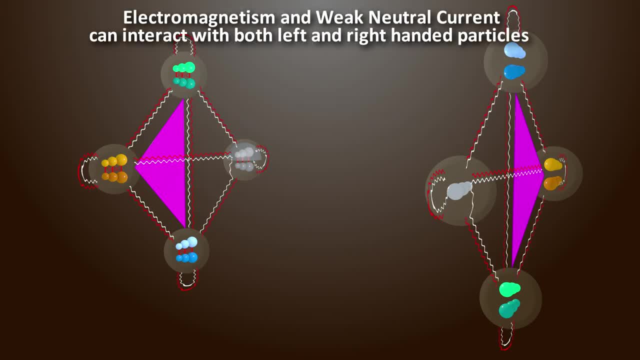 Also note that, unlike the charged weak force, the neutral weak and electromagnetic forces can interact between both left and right-handed particles. This is because the neutral weak force and the electromagnetic force appear to come from a single force that existed near the universe, called the electroweak force. I have a video on this if you want to know more details. 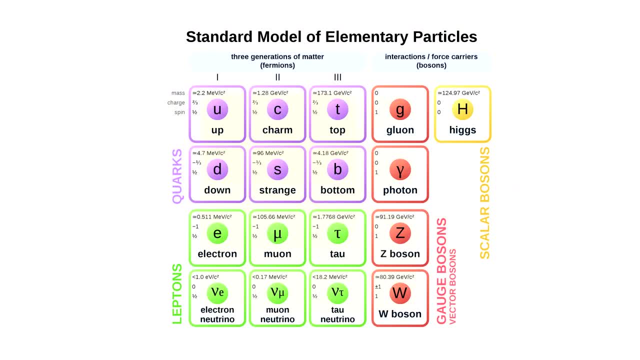 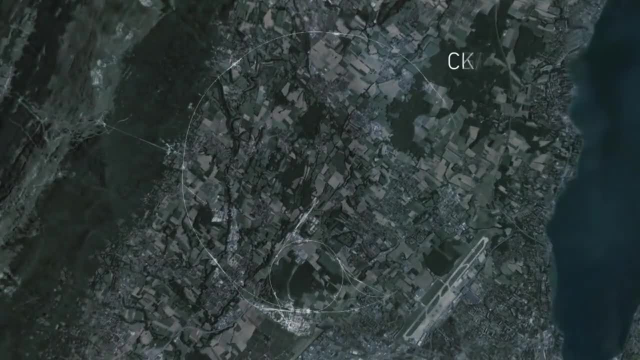 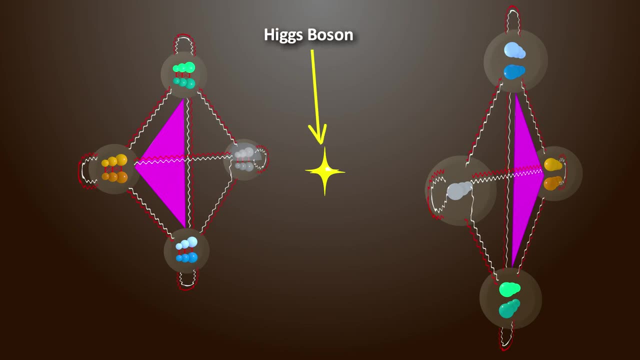 At this point, we've discussed all particles except one critical one, The grand poobah of fundamental particles that was predicted more than 50 years ago but only confirmed in 2012 at the Large Hadron Collider in CERN, Switzerland. That particle is, of course, the Higgs boson. This 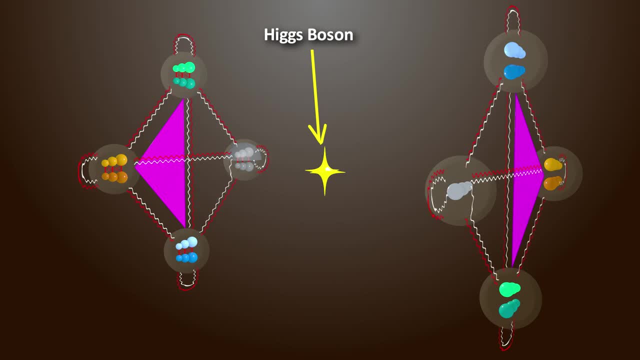 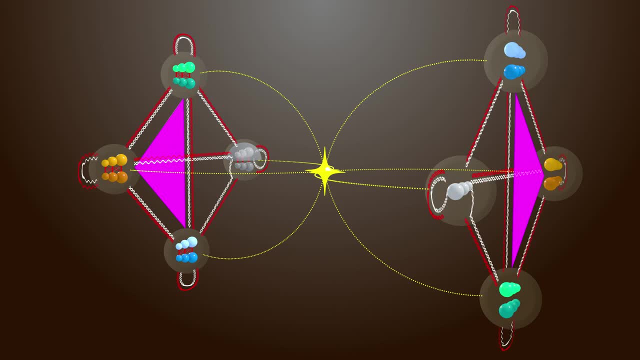 the mass of a particle. The Higgs boson connects to all of them, But there is one exception: the neutrino. The Higgs does not interact with them according to the standard model. So how neutrinos acquire mass remains a mystery. 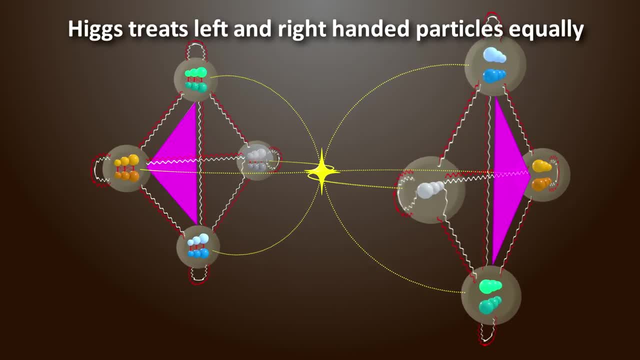 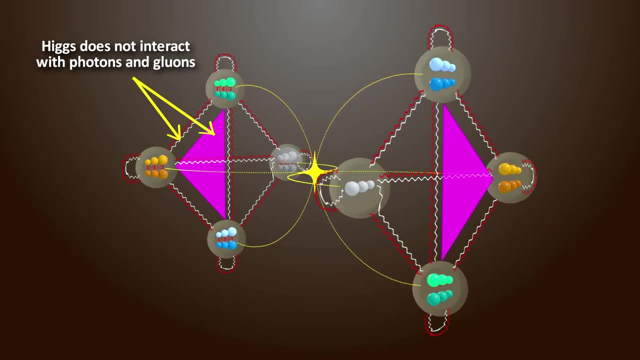 The Higgs particle doesn't care about right and left handedness and treats both equally. The only bosons that do not interact with the Higgs are the gluons of the strong force and the photons of the electromagnetic force. These two particles thus have zero mass. The amount of mass conferred to these fundamental particles depends on how much they interact with the Higgs field. The greater the interaction, the higher the mass. So, for example, the top quark interacts more with the Higgs field than the charm quark, thus gains a higher mass. 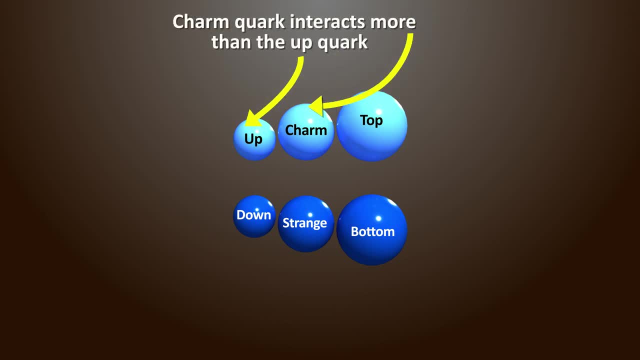 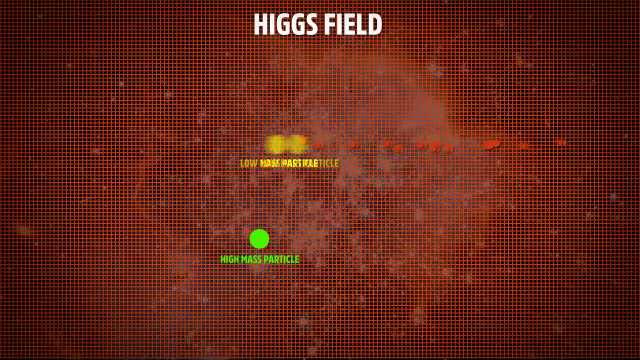 Likewise, the charm quark interacts more with the field than the up quark, so it has a higher mass than the up quark. For simplicity, you can think of this interaction with the Higgs field as slowing the particle down. The more the interaction, the slower the 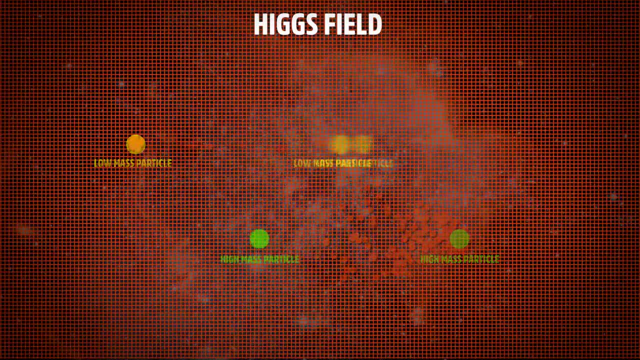 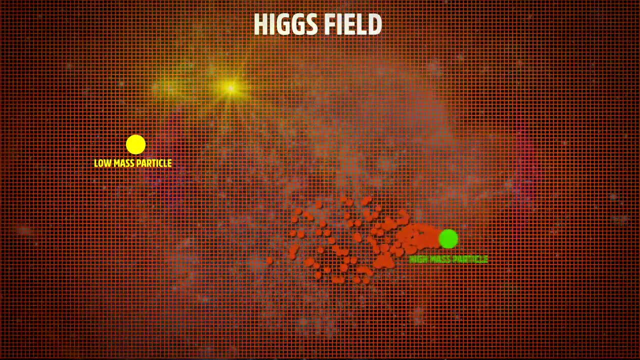 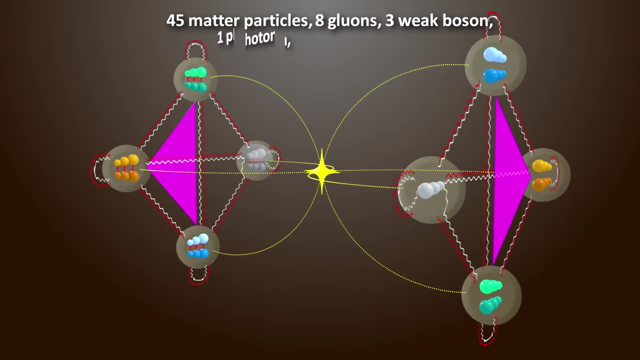 particles become and the more mass is conferred. Massless particles, like photons, do not get slowed down and so travel at the maximum speed allowed by nature: the speed of light. So the final count is the following: 45 matter particles, 8 gluons, 3 weak bosons, 1 photon. 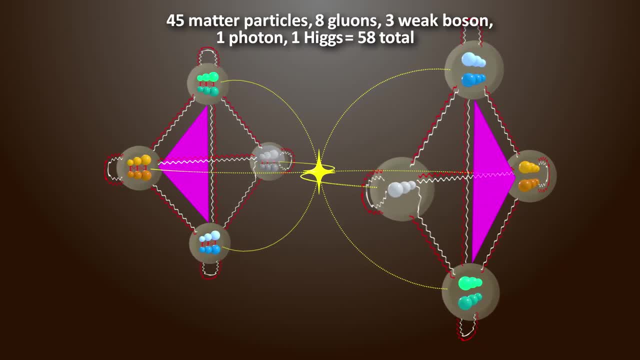 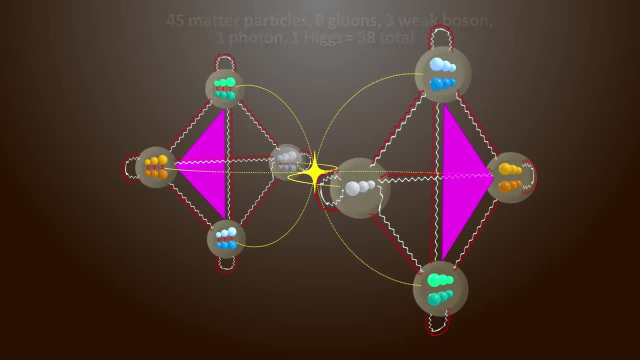 and 1 Higgs particle. In total, 58 particles with different handedness, charges, colors and interactions. This is a full picture of the standard model of particle physics, but you shouldn't be surprised if you don't know that the mass of a particle is equal to the mass of a particle. 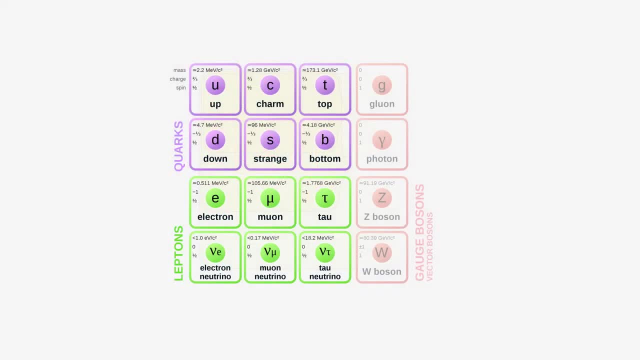 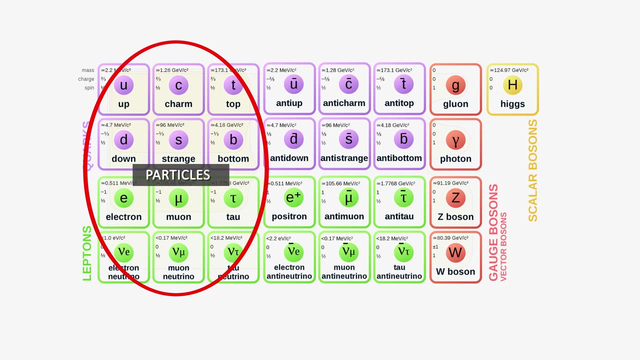 You should know that this is not the end of the story. While we have 58 particles, we also have an equivalent amount of antiparticles. Antiparticles are generally the same as regular particles, except they have opposite properties, such as charge. So, for example, the antielectron. 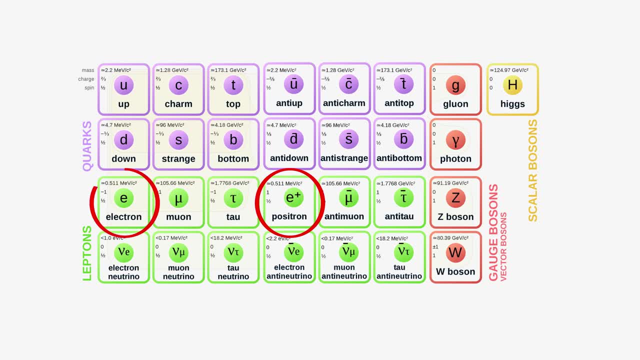 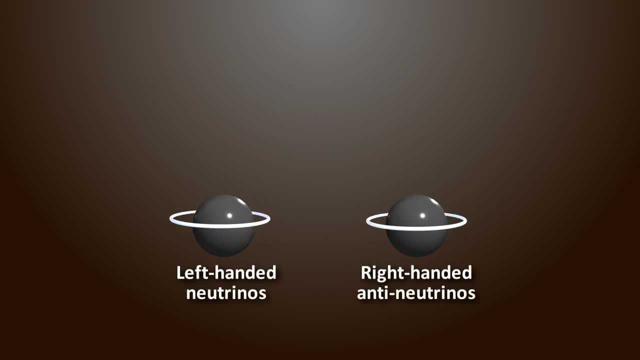 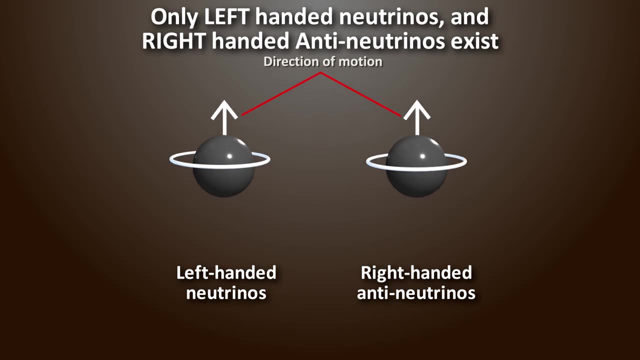 called a positron has a positive charge, whereas the electron has a negative charge. Handedness also changes. So, for example, antiparticles of left-handed particles are left-handed. This means that while only left-handed neutrinos exist, only right-handed antineutrinos.